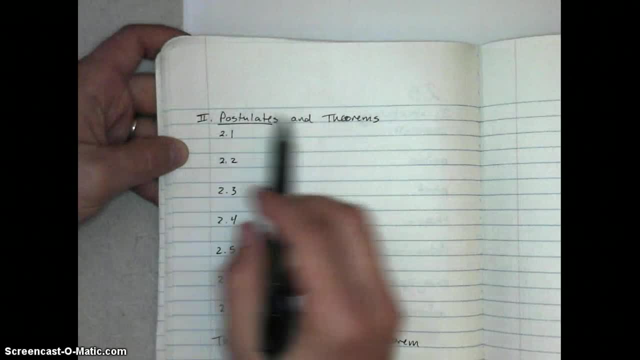 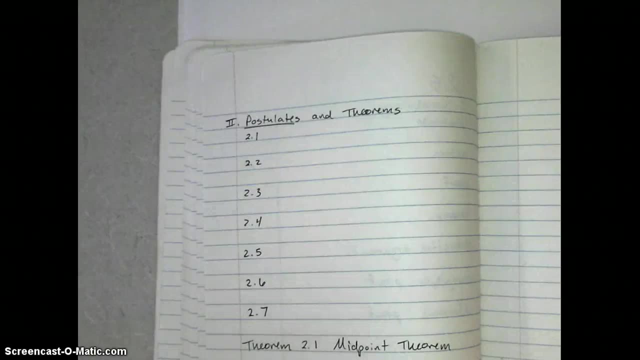 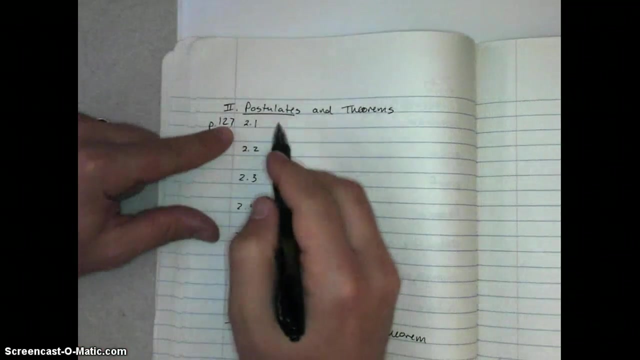 We wanted to talk about postulates and theorems. There are no properties in this lesson, so we'll just say postulates and theorems. The first seven can be found on page 127.. And they don't have what we call proper names. 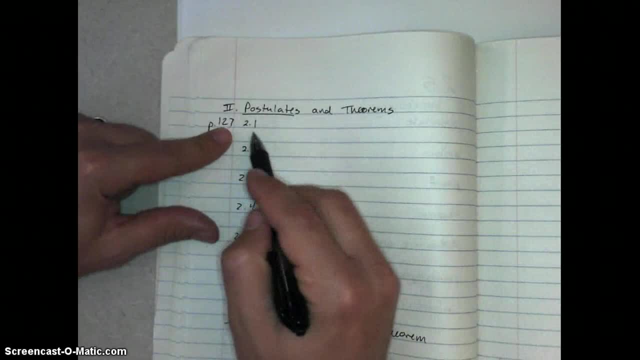 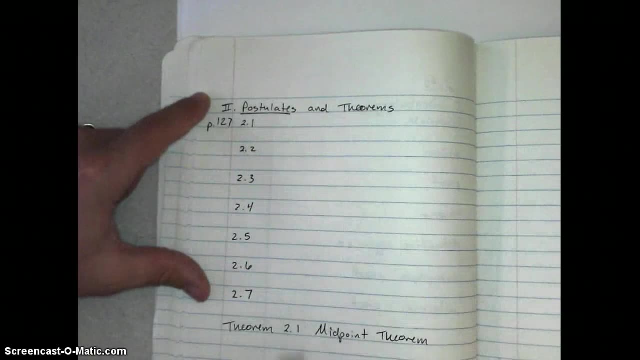 They are just written out in sentence form after this number. This identifying number is only really good for our book. Each book can title them a little bit different, And so these postulates need to be written out most of the time. But then we do have a theorem- 2.1, that has what we call a proper name. 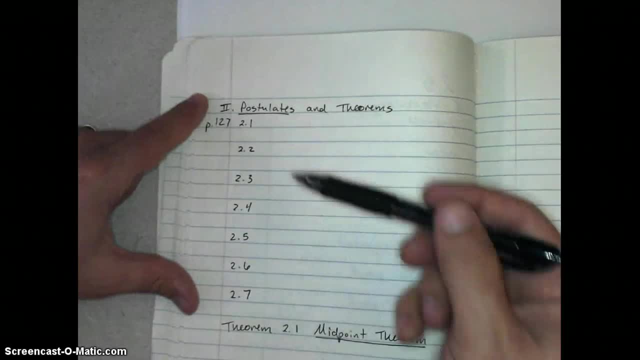 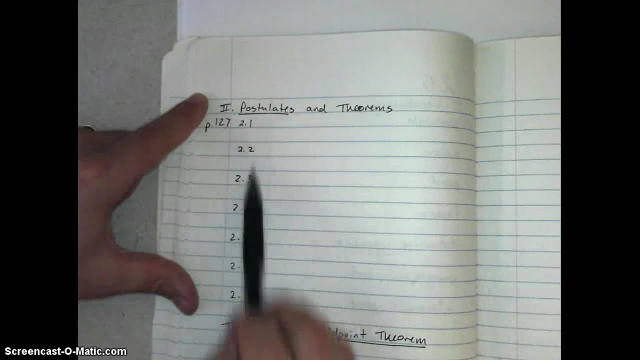 It's called the midpoint theorem that we'll get to later in the lesson. So when you're writing these down, if anything were to ever have a proper name, go ahead and write that and underline it like I've done here. But for all these postulates, we can just refer to them by their number and then write them out in your vocab book. 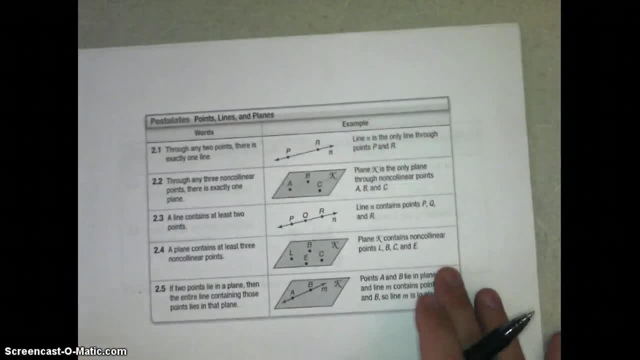 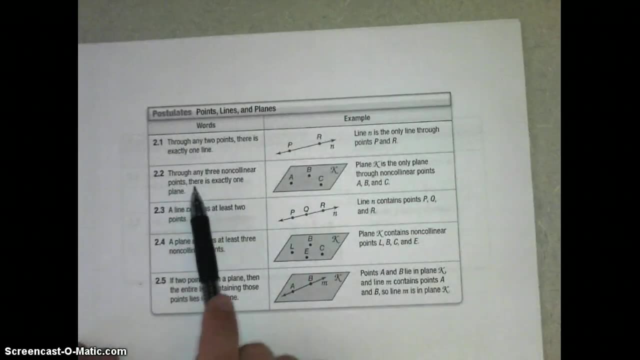 Alright, let's go ahead and take a look at those real quickly. You should have these postulates written down Through any two points. there's exactly one line. The next postulate is through any three non-collinear points. make sure you have specified non-collinear. 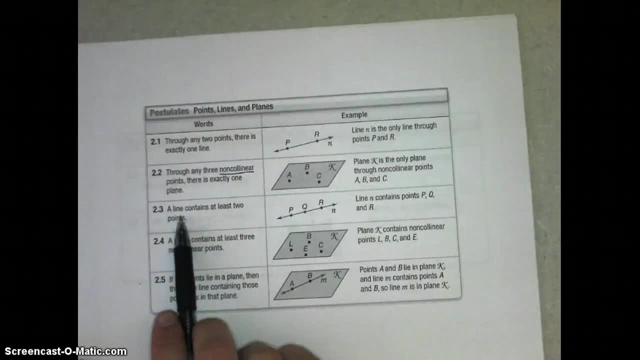 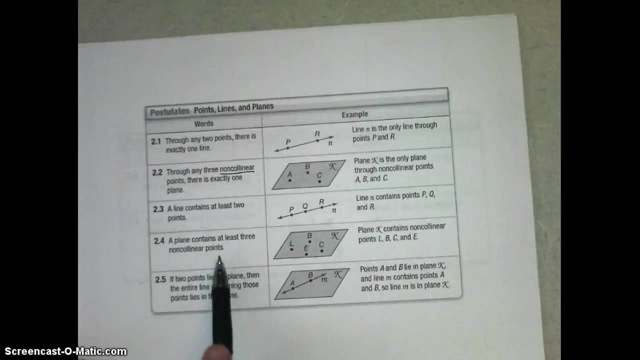 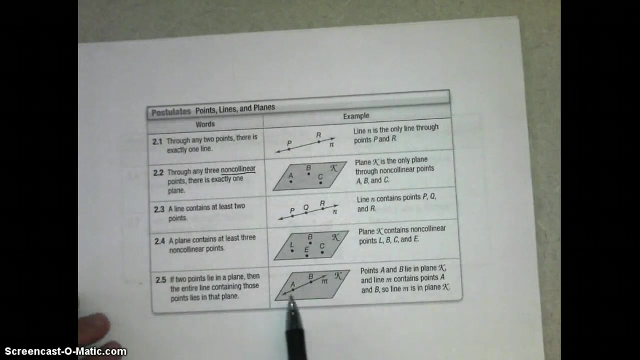 there's exactly one plane. A line contains at least two points. That's a postulate. Another postulate is that a plane contains at least three non-collinear points. These postulates kind of come from the first two And then next, if we have a plane. 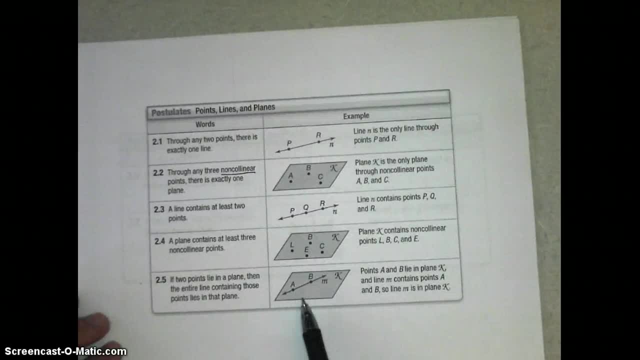 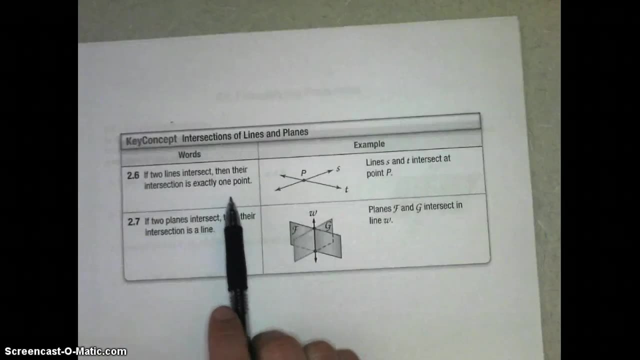 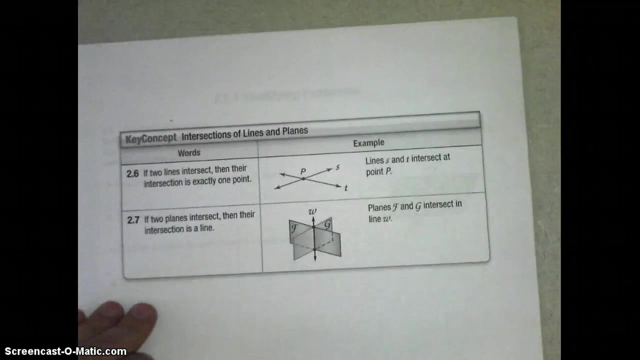 and two points lie in that plane, then the line containing those two points also lies in that plane. Then our last two postulates: if two lines intersect, then their intersection is exactly one point. And to seven: if two planes intersect, then they intersect in a line. 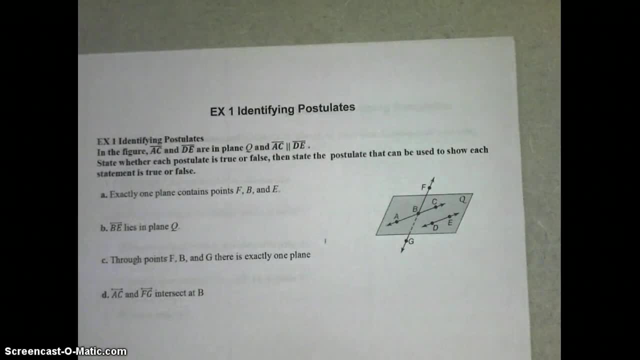 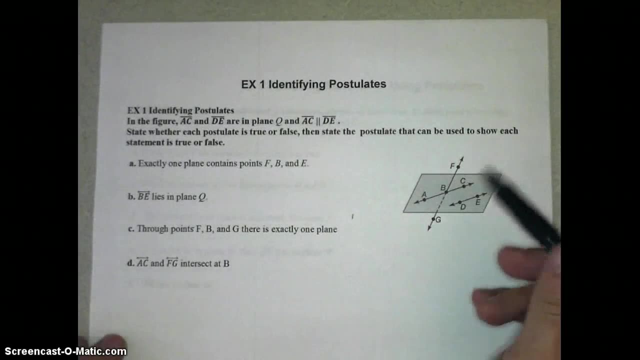 So we're going to use these postulates, which are these mathematical ideas that do not have to be proven to be true, They just are accepted as true without proof, And we're going to use those to help us justify some statements here. So let's look at example 1a. 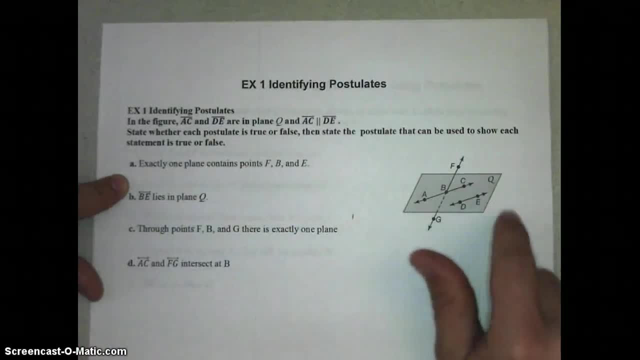 In this figure we're told that AC and DE are in plane Q and they're parallel. So we should be able to state whether each of these postulates is true or false and identify that postulate from your list that makes them true or false. 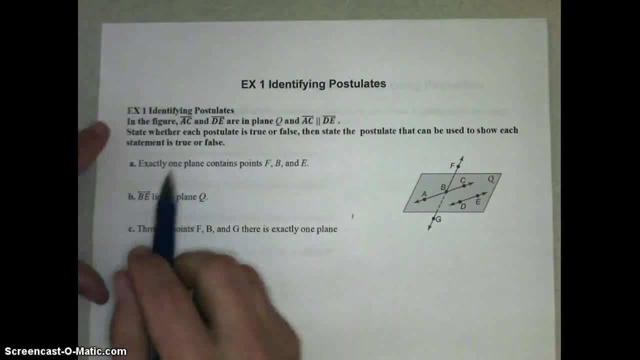 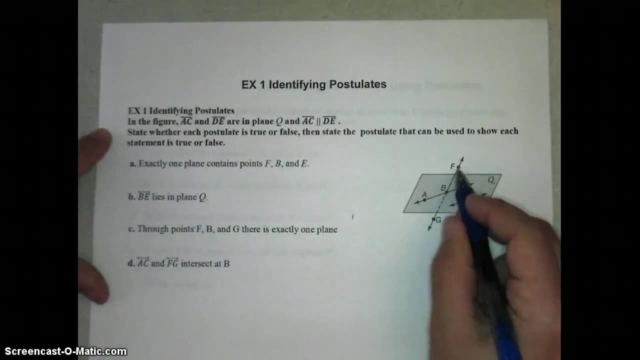 So let's take a look at number 1a. Exactly, one plane contains points F and B and E. Well, we have F, B and E. Those are non-collinear, Even though F is above that plane. these are three non-collinear points. 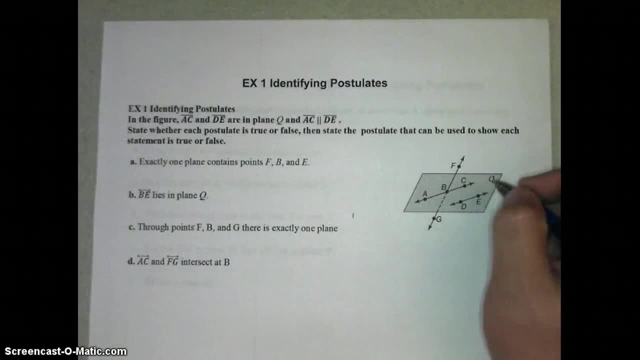 And we have a postulate that states: through any three non-collinear points there's exactly one plane. Also, we have the one that says a plane contains at least three non-collinear points. But that first postulate- 2,, 2, is what tells us this. 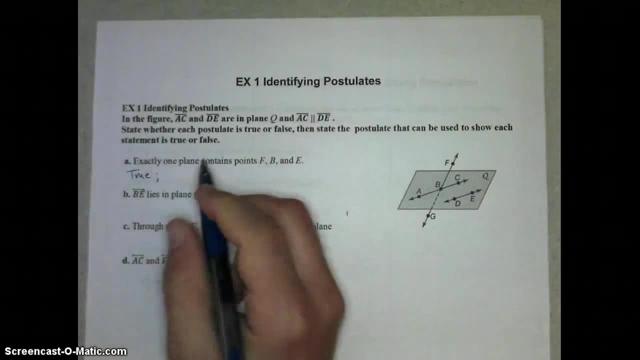 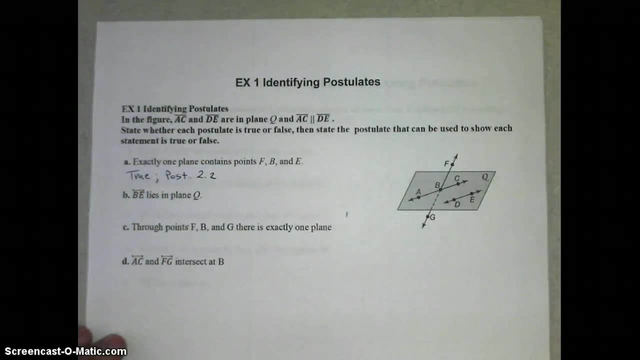 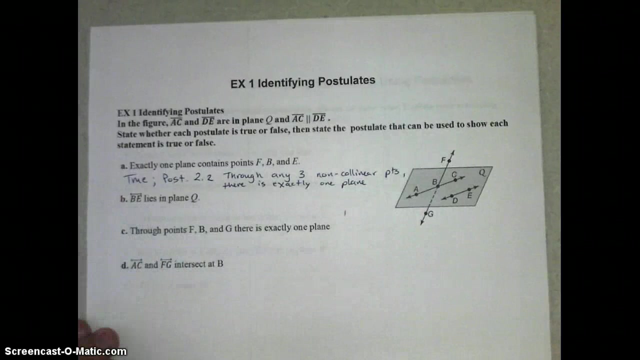 So this is true because of postulate. you can abbreviate this 2.2. which states: through any three non-collinear points there's exactly one plane Part. We have line BE and we're told that BE. 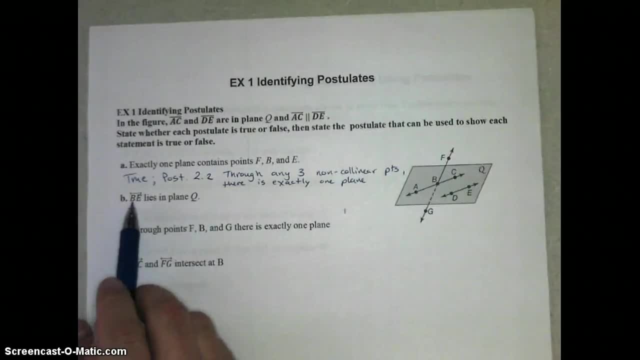 even though it's not drawn. if there's two points, we get a line, that line lies on plane Q. Well, since BE and E are both in plane Q, the line containing those two points is also on plane Q. So that is true. 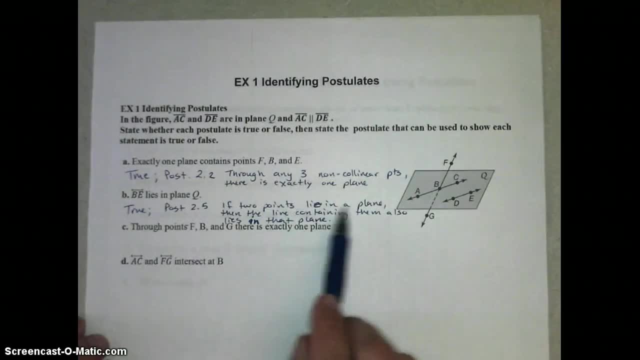 By postulate 2.5.. if two points lie in a plane, then the line containing them also lies in that plane. Why don't you try parts C and D, see if you can identify if these are true or false statements and write out the postulate? 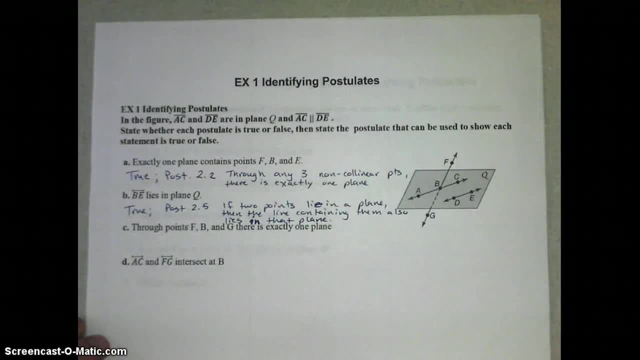 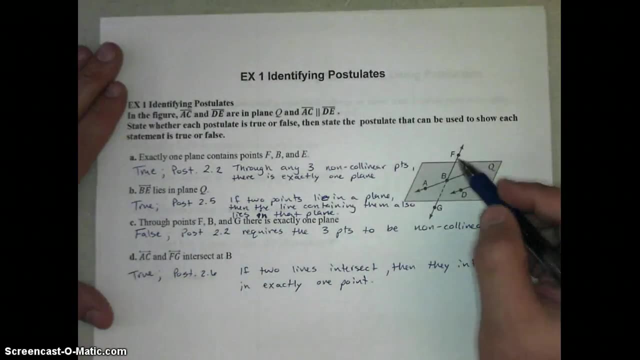 that makes those true or false. Alright, this is what we should get For part. it says: through points F, B and G there's exactly one plane. The problem is that F, B and G are collinear. 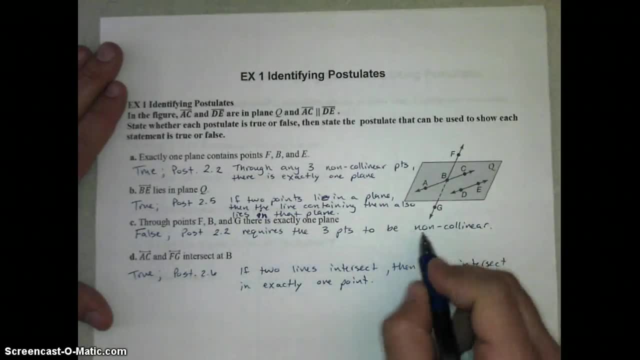 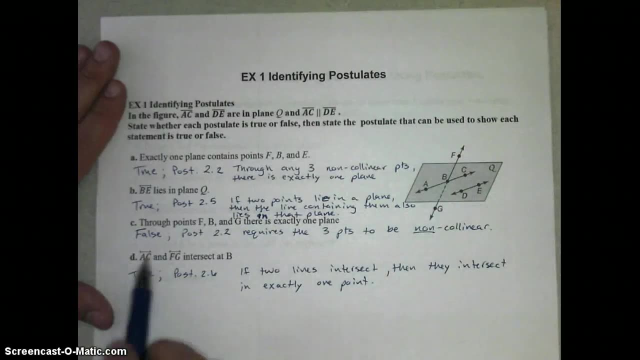 and postulate requires the three points to be non-collinear. So this is actually false. There's more than one plane containing those three points. Part this is true. We're told that AC and FG intersect at B If you look at the diagram. 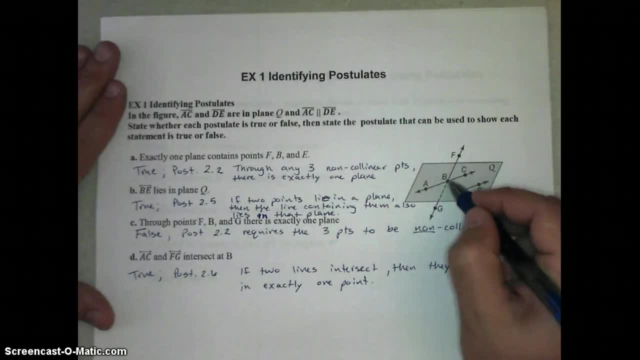 AC, FG do intersect and the point of their intersection is B, and since postulate states if two lines intersect, then they intersect at exactly one point, this is true. Alright, in table we're doing some of the same kind of stuff. 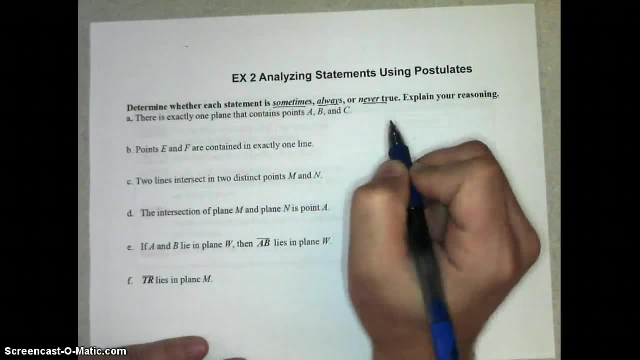 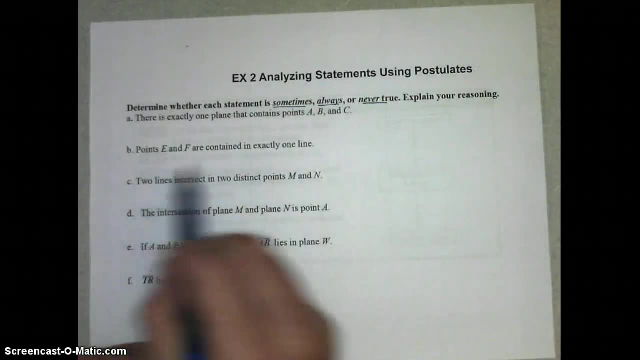 but these could be sometimes always or never true, and we don't have a specific diagram to look at, and so we are just making general statements about these points that exist somewhere, but we don't actually see them in a diagram. 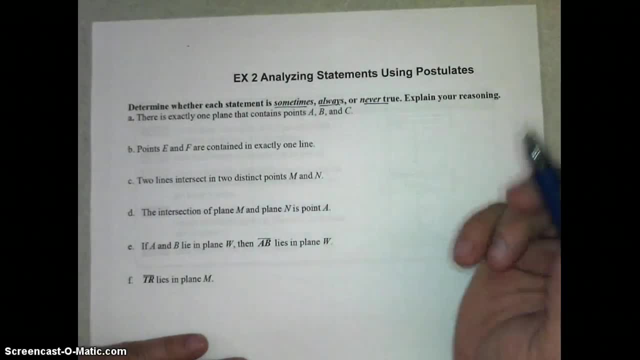 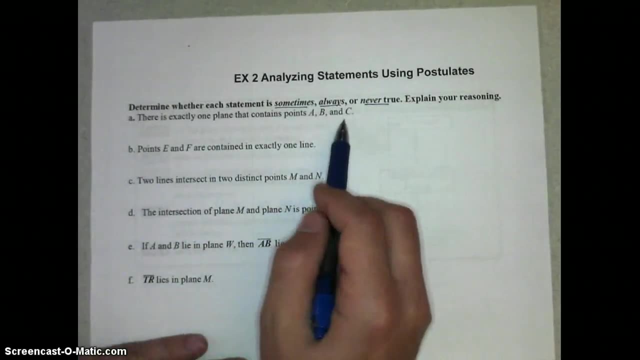 We are to explain our reasoning again by citing some different postulates. So let's take a look at There's exactly one plane containing points A, B and C. Well, without knowing any more about these, this could be true or false. 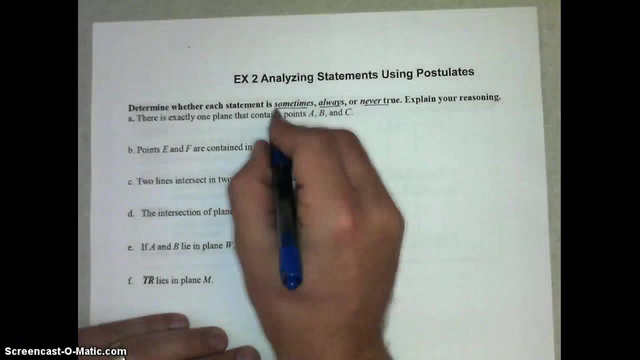 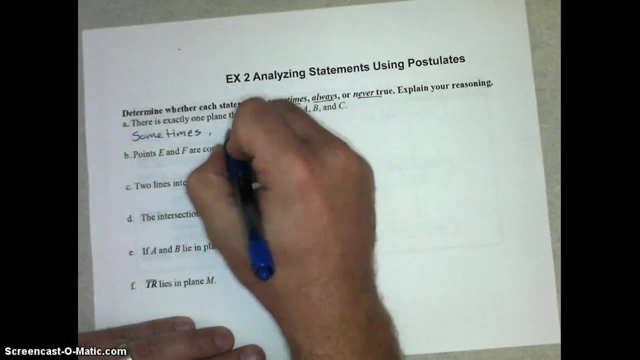 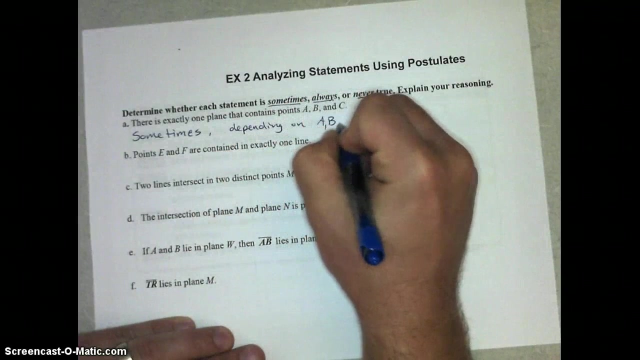 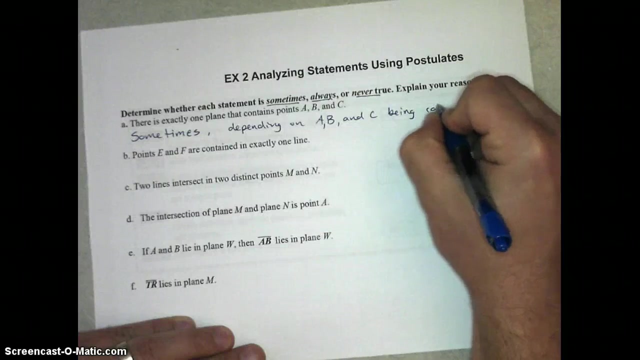 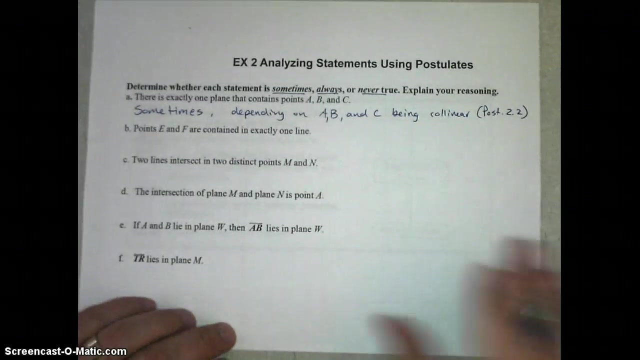 depending on whether A, B and C are collinear. So this is a sometimes true And it depends on whether or not A, B and C are collinear, And that's postulate. Next, points E and F are contained in exactly one line. 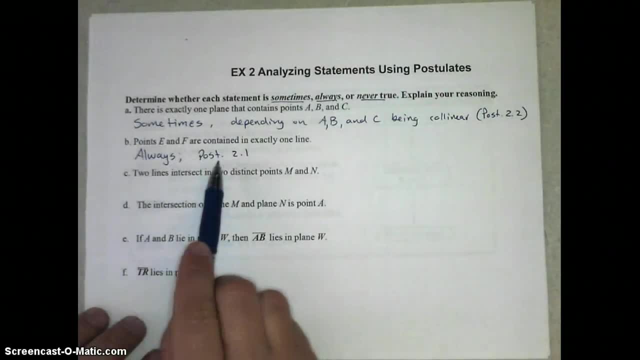 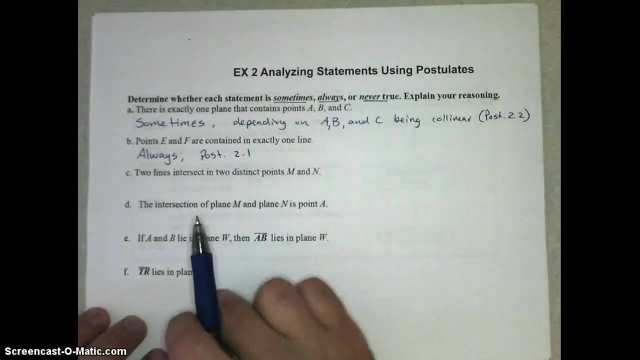 This is always true because of postulate. Through any two points, there's exactly one line. Why don't you try through on your own and then, when you are ready, you can continue watching the video to check your answers. 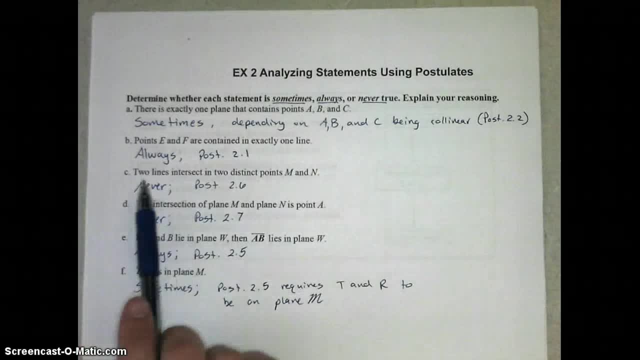 Alright, here are the answers we should get. If we have two lines intersecting in at all, they intersect in exactly one point. So this is never true by postulate. Part says the intersection of plane M and N is a point. 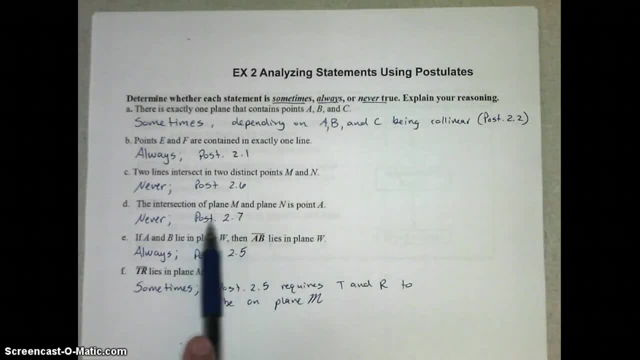 Well, that's not true because of postulate: If we have two planes intersecting, they intersect in a line, not just a point. So that's never true Part. if A and B lie in plane W, then line A B lies in plane W. 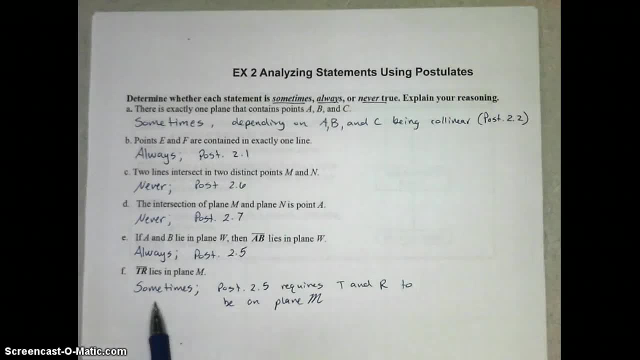 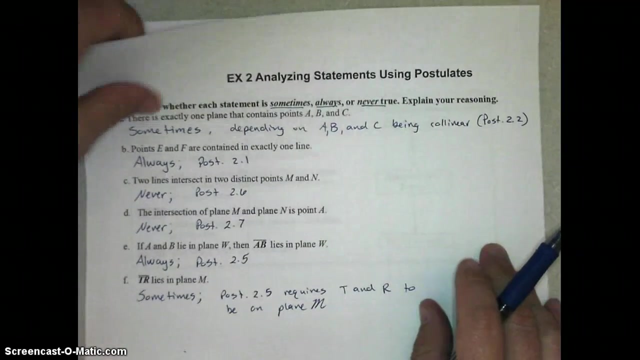 That's always true by postulate, And similarly part, if T, R is to lie in plane M- that can sometimes be true- Postulate requires that T and R, both of those points, must be on plane M. Alright, let's take a look at the proof process. 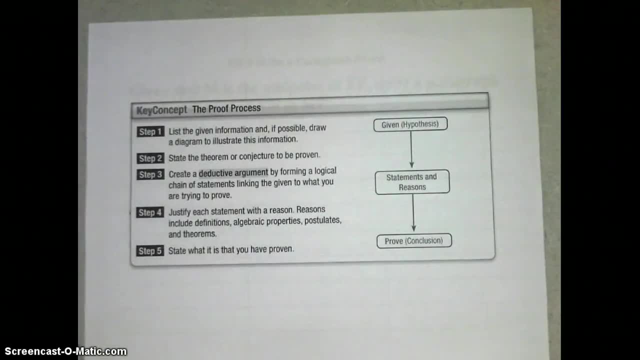 In writing proofs and kind of using these postulates and properties and things like that to help make arguments, our deductive arguments. there are five steps we must go through. First, we need to list the given information and, if possible, draw a diagram to illustrate that information. 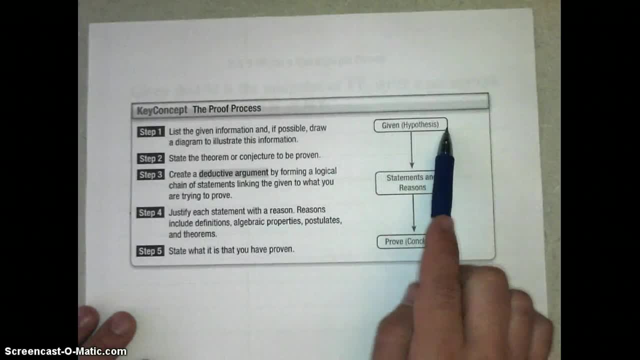 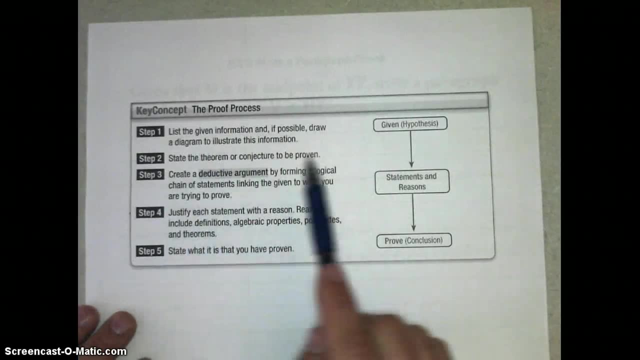 Okay, and that's where we are given our statements. That's like our hypothesis. Step two is to state the theorem or conjecture to be proven, And a lot of the times we'll put both of these pieces together And then, in step three, we can create our deductive argument. 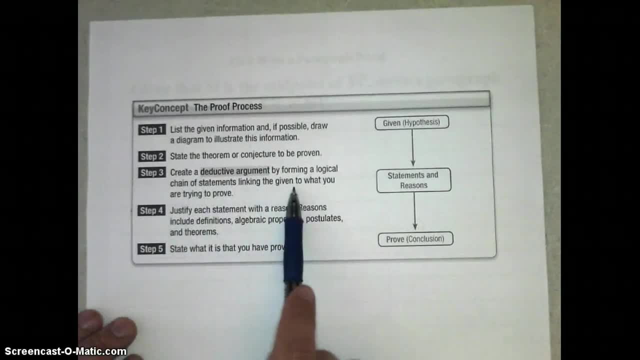 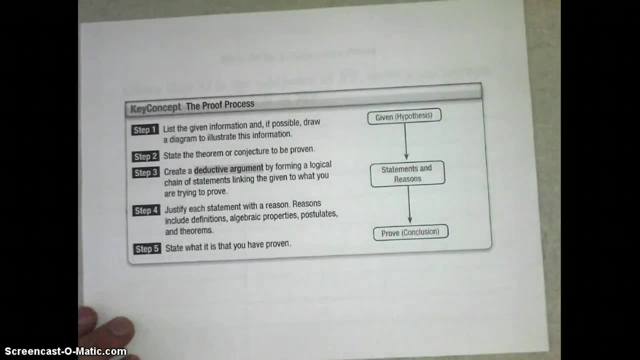 by forming logical chain of statements linking the given to what you are trying to prove. We want to create a chain that is linked together. I can't skip links in the chain of logic without summing those up. In step four we're going to justify every statement we make. 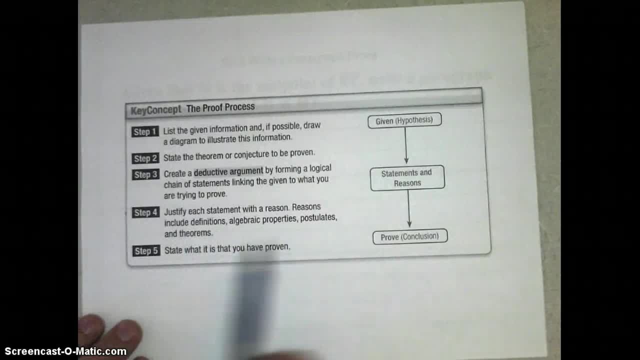 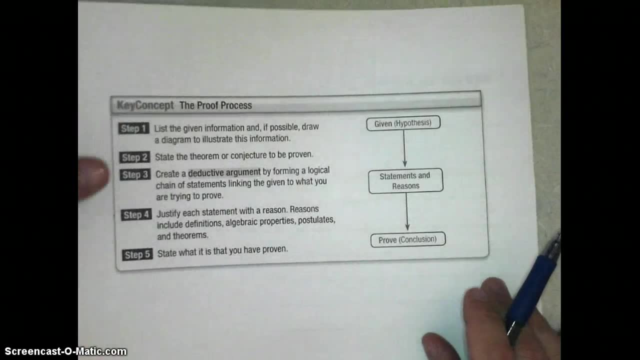 to including definitions, algebraic properties, postulates and theorems. And, lastly, we're going to state what we were trying to prove as proven. So we're going to keep this in mind as we try and construct our proofs. 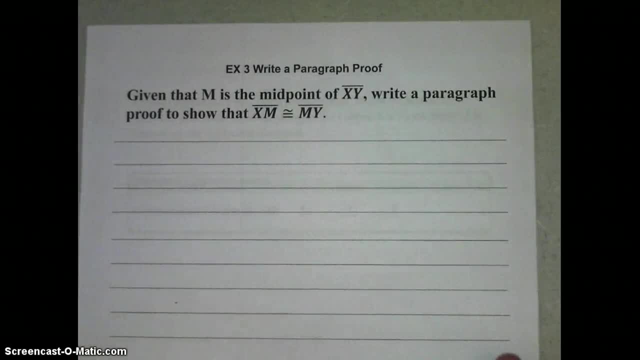 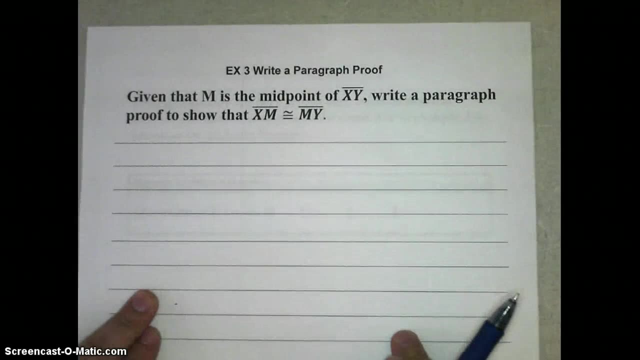 And in lesson two six, you learned how to put together two-column proofs for algebraic proofs and geometric proofs, in which you list your statements on one side, reasons on the other. But a lot of times it's a little bit easier. 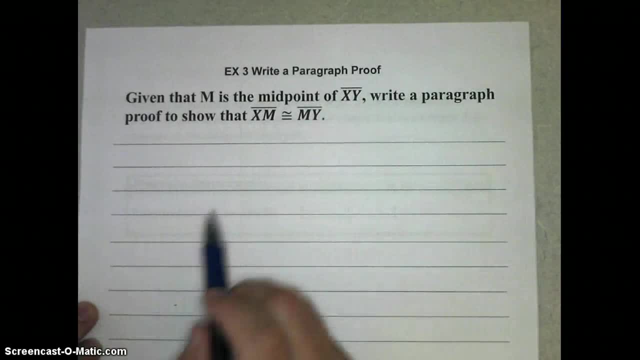 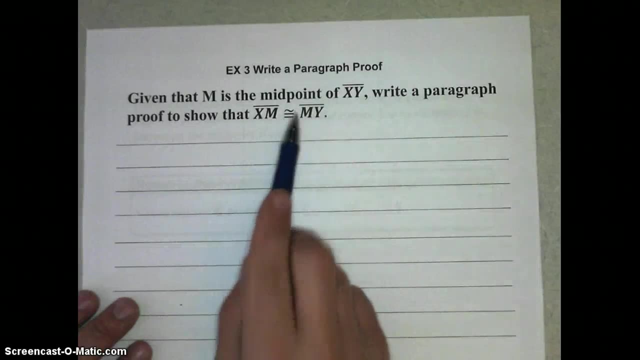 just to write out your proof in paragraph form. So this is how we're going to do that. We're given that M is the midpoint of, We need to write a paragraph proof to show that XM is congruent to. So the first thing we need to do in our proof process, 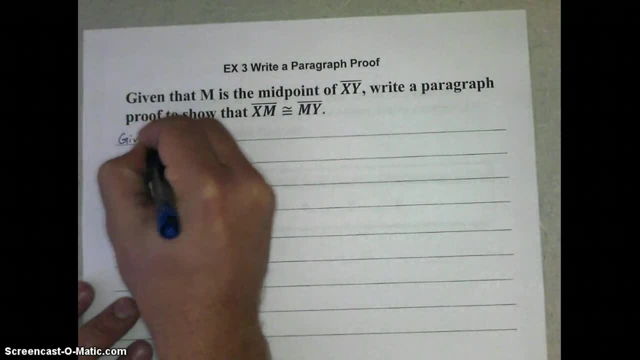 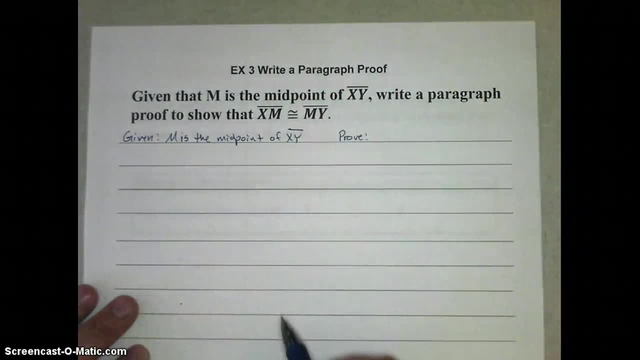 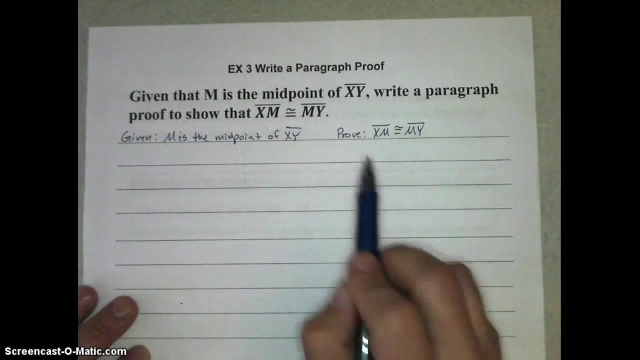 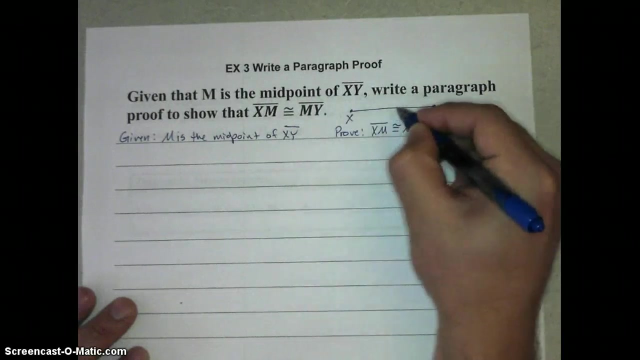 is state the given M is the midpoint of, And state what it is that we're trying to prove. XM is congruent to Now. a lot of times it's good to put a diagram with that. So we know from our diagram these have to be congruent. 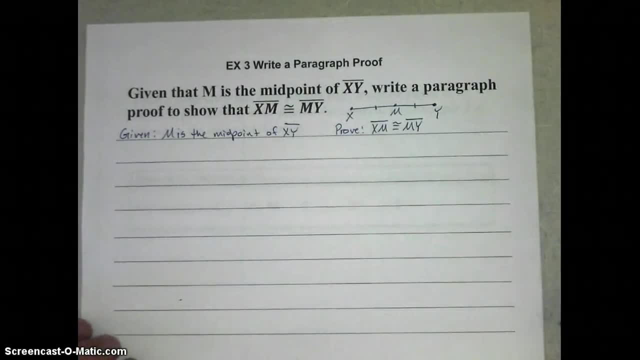 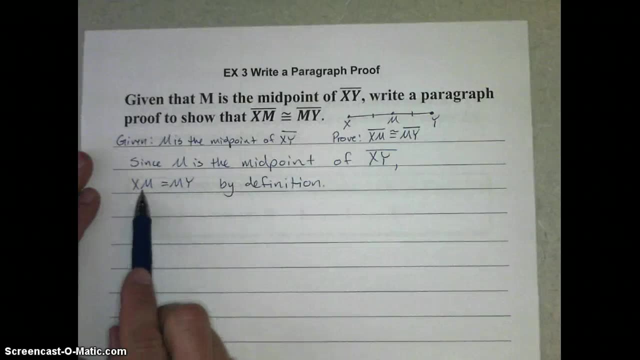 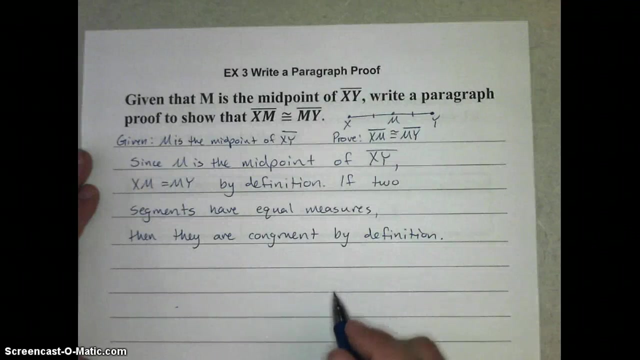 We just have to be able to explain that. So here's how we're going to put that in paragraph form. Our first sentence can read like this: Since M is the midpoint of XM equals MY by definition, And since we know that these are equal, 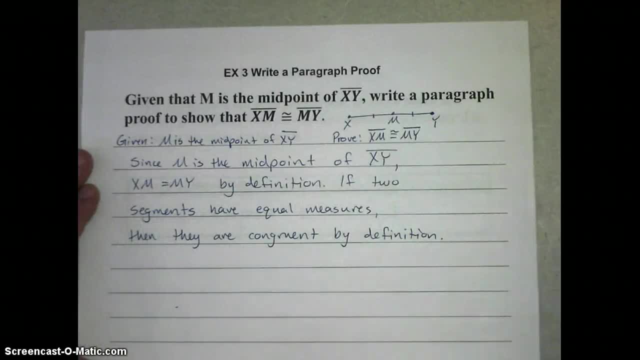 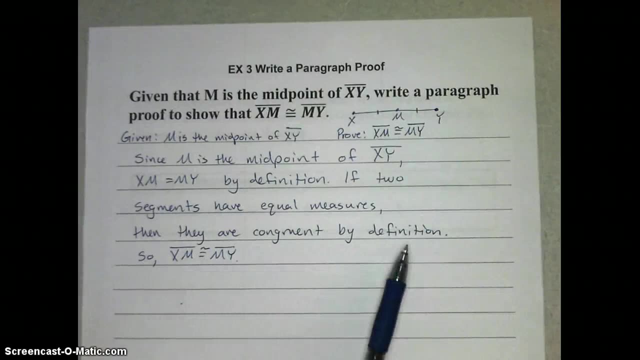 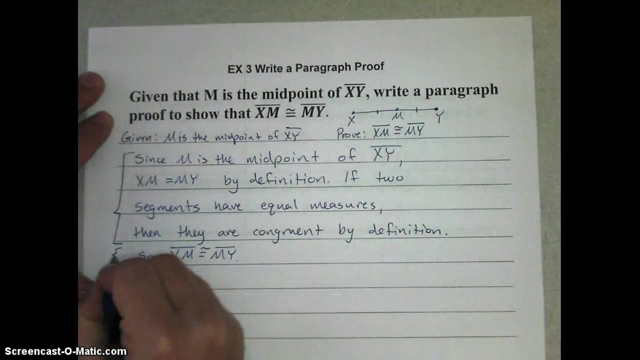 if two segments have equal measures, then they are congruent by definition. So XM is congruent to MY- And I've already given my reason before that- And so this is the body of the proof. And then we have finally proven what we set out to prove. 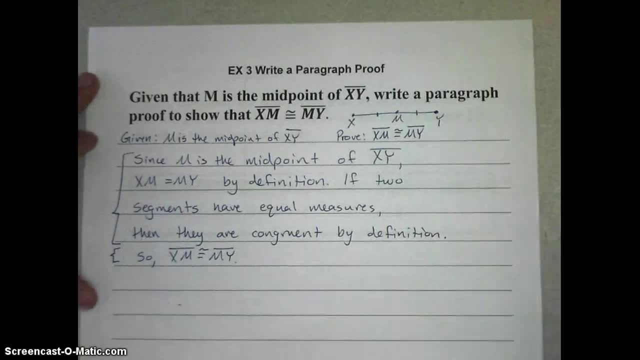 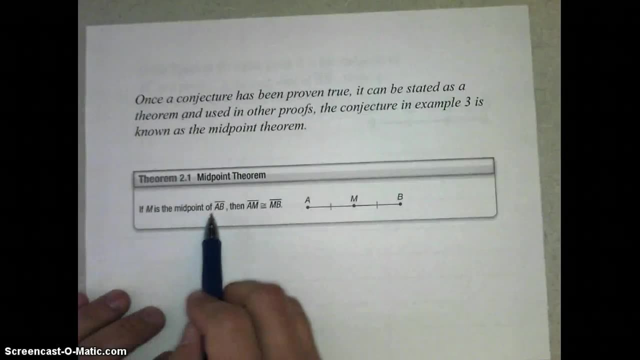 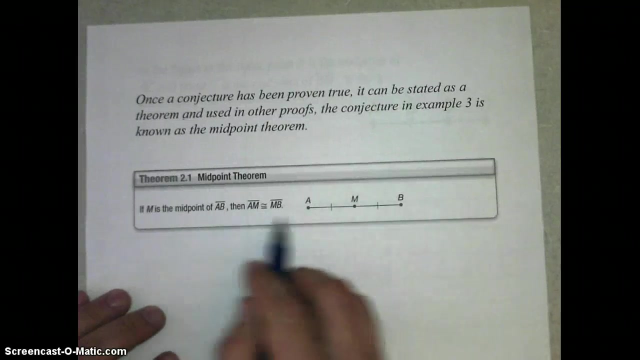 in that final statement, But it all fits nicely in one paragraph. Now that proof helps us explain this theorem. If we have M as the midpoint of a segment AB, then AM is congruent to MB. This is not our definition in the strict wording. 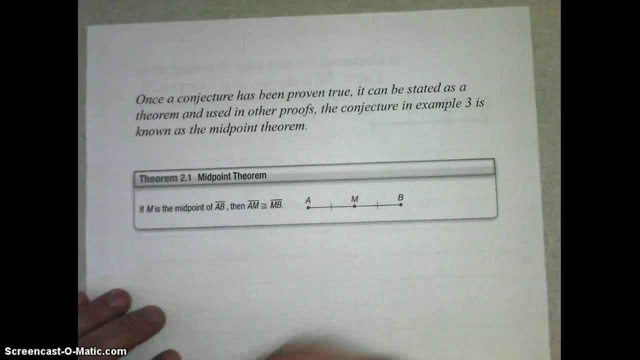 that we were given earlier in this course for midpoint, But we've gotten this information from that definition, And so this is what a theorem is. Our theorem comes from other postulates and ideas and definitions and is a new idea that we can now move on and use in other proofs. 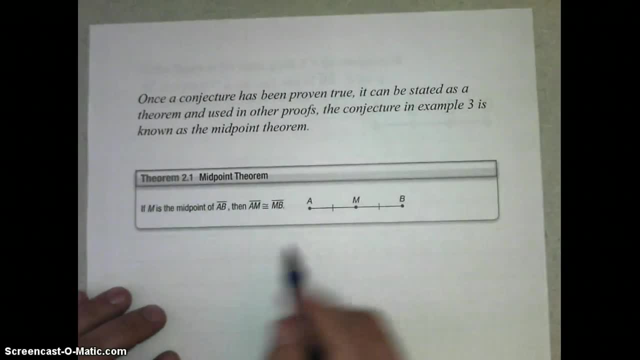 So now we have the midpoint theorem. We just proved that in example 3.. So we can use that theorem in other proofs. Whenever we're told that we have a midpoint, we can make a conclusive statement like this because of this theorem, And so this could be a reason in a proof. 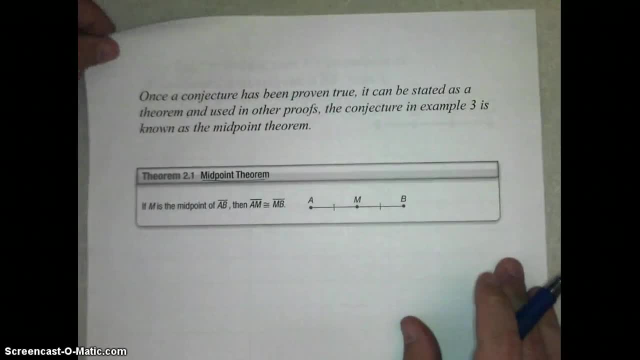 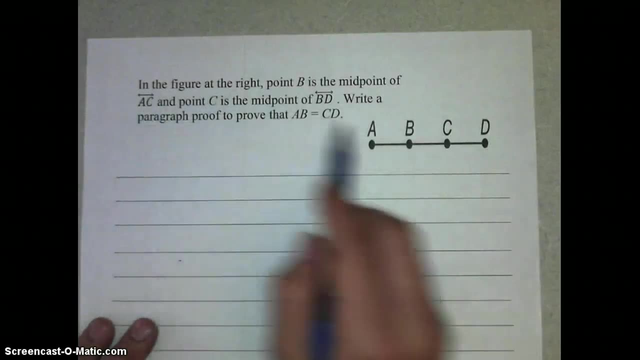 The midpoint or a reason in a proof, The midpoint theorem. Alright, so we've got one more example to try. If we're given this diagram and we're given that B is the midpoint of AC, go ahead and mark the diagram like that. 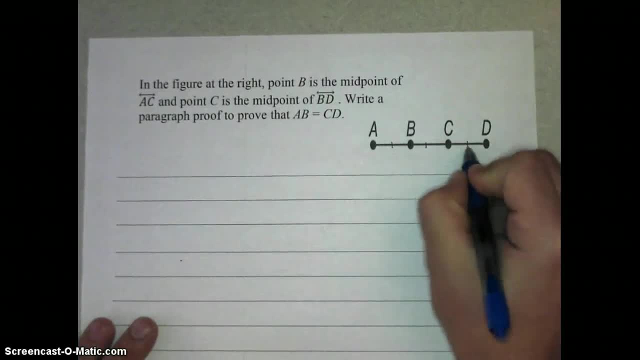 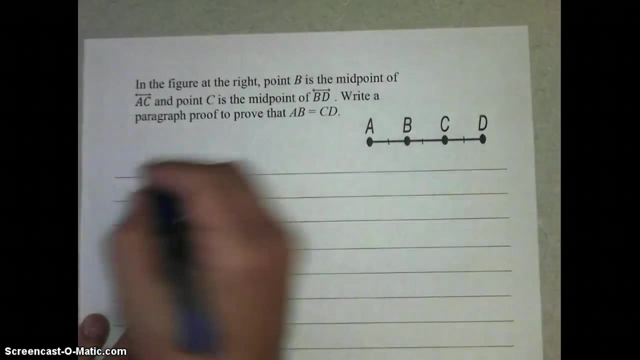 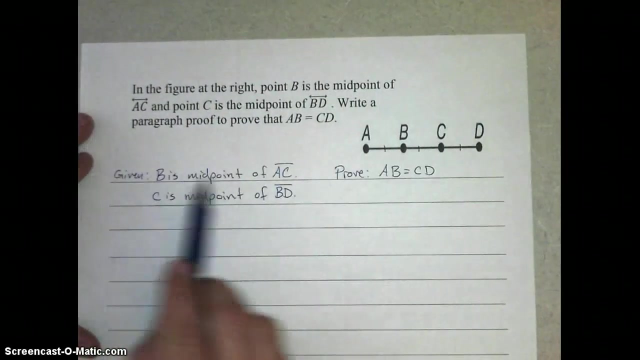 but also C is the midpoint of BD. so we can mark all three of those like that. we should be able to prove that AB equals CD. So I want you to take a look at that. The given information is this: B is the midpoint of AC and C is the midpoint of BD. 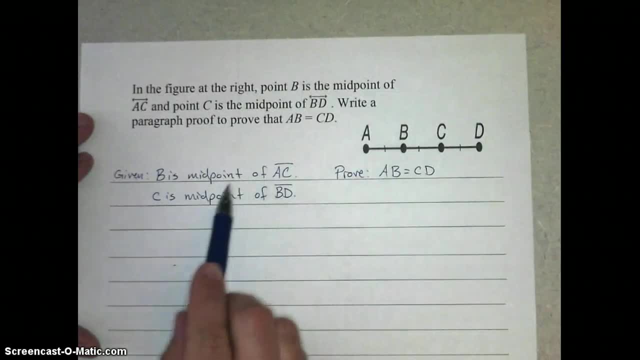 and we're supposed to prove that AB equals CD. Notice, we're talking about midpoints, talking, then, about the equality of their lengths. So here's how we should start our proof. We want to begin by just stating the given, Since B is the midpoint of AC and C is the midpoint of BD. 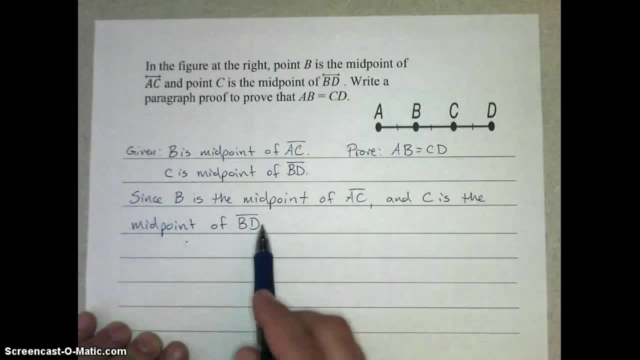 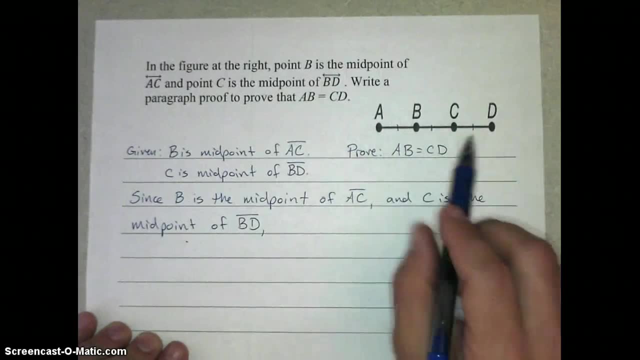 notice. I'm using the word since because in my sentence I'm going to imply that something else follows that. Since I know that B is the midpoint of AC and C is the midpoint of BD, I can make another statement to eventually lead me to something.